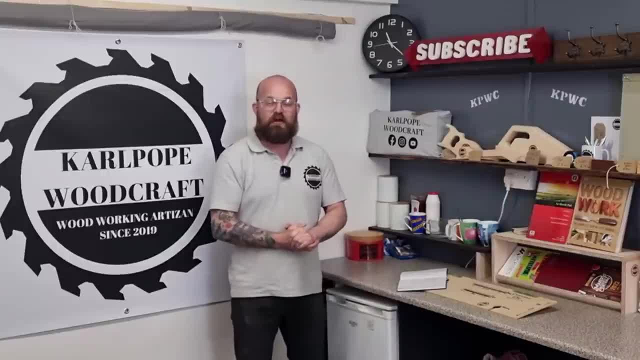 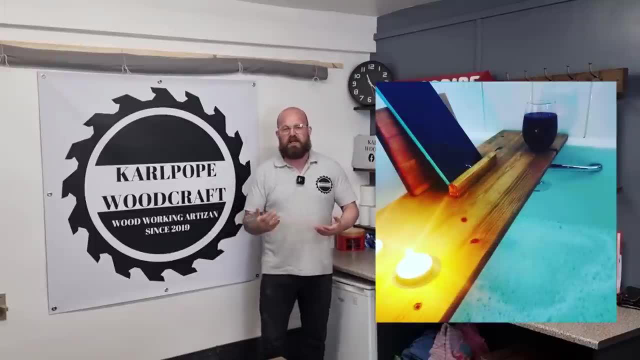 themselves, so you get a visual uh representation of what they look like as well. number one, then: what tools you're going to need to make at the bath caddies, you're going to need a drill, some type of saw, whether it be a hand saw, a jigsaw, a mitre saw. you're going to need a sander- random. 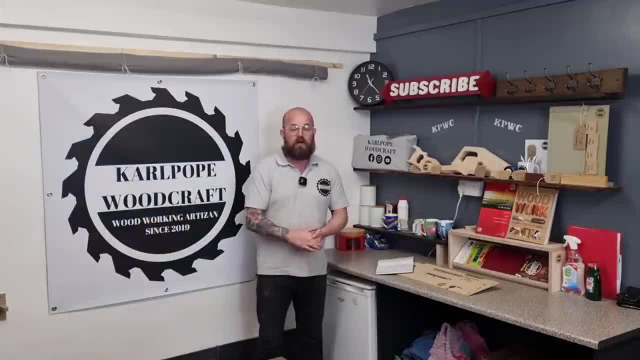 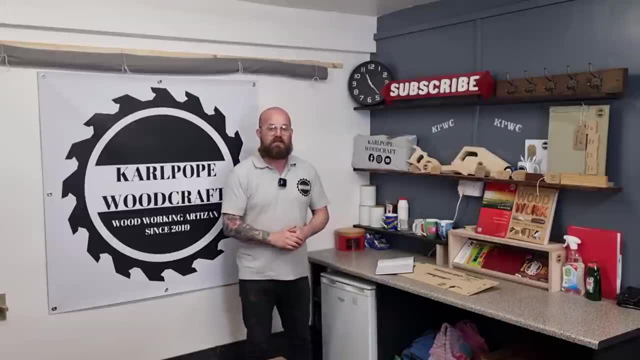 orbital sanders best, but if you've got one of them, little mouse sanders that'll do, or even by hand, that's totally fine as well. one of the best ways to reproduce the item is to use a template. so for the bath caddies we have these templates. they're really simple to make. they're made out of six. 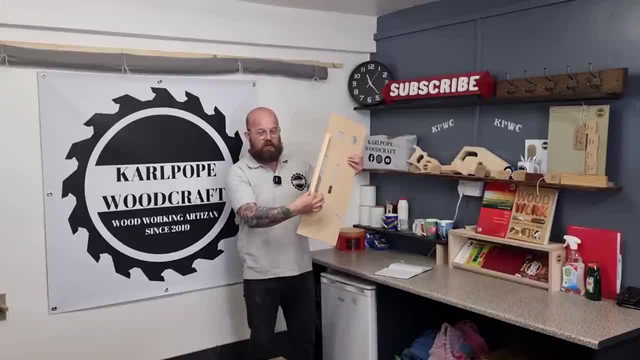 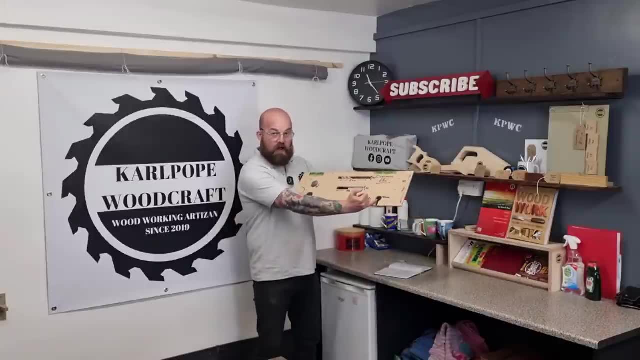 millimeter mdf, a little piece of paper, and then we're going to take a piece of paper and we're going to take a piece of pine strip on the back so you can hook it onto the piece of wood, and on the front you have the layout of where you're going to have the candles, where the wine glass is going to. 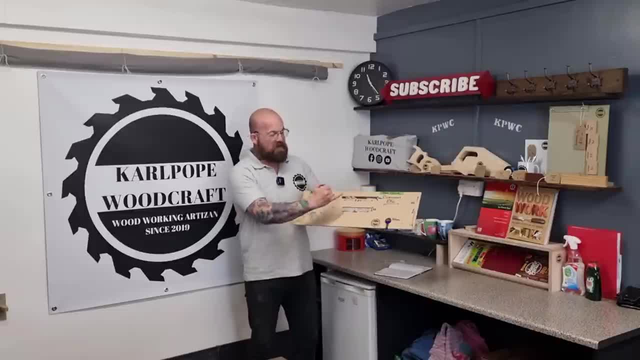 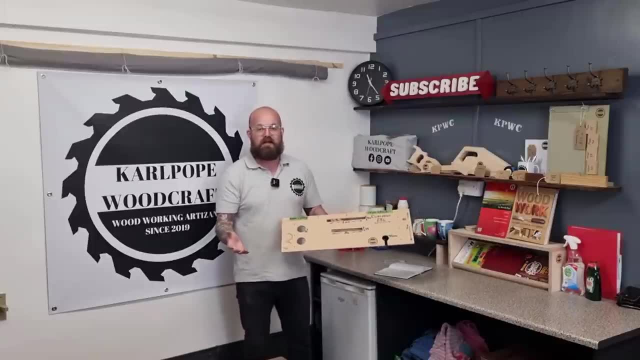 go and the little holders for your laptop or your phone, and we also have the dimensions on here where screws are placed and things like that. that way you can reproduce it without having to work out your plan every single time. templates are definitely the way forward when you're wanting. 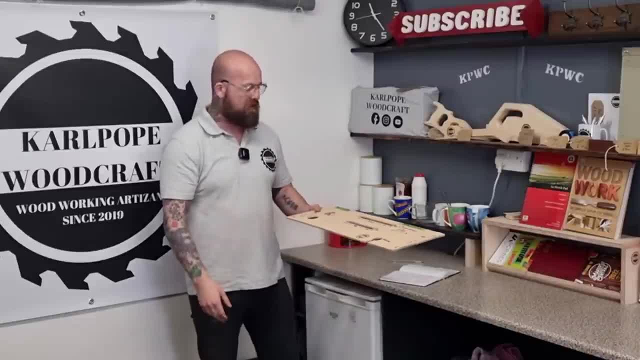 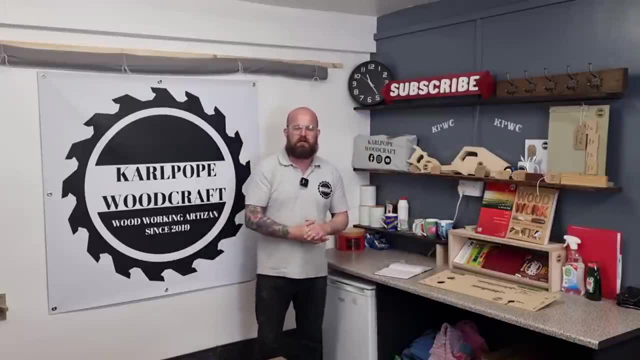 to make something over and over again and make money at doing it as well. right then, these these elements. i just started feeling way better now because we're going to have thehing in a bit, but for a couple weeks, i think, if you're taking one about three days off and you're creating. 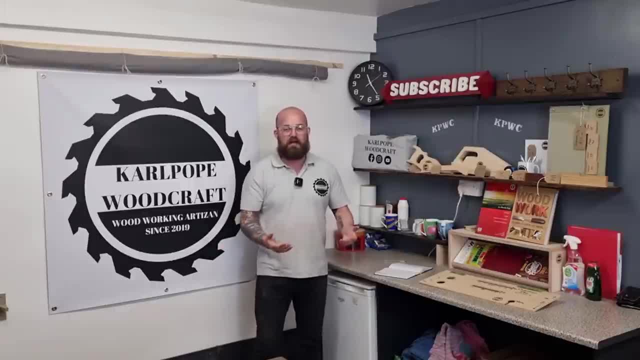 one of the real materials. totally, it sounds pretty cool. so all of our plans are: number two are going to be your, something that you get for you. you're going to top it off a couple of dollars, depending on the area where you are. they might go down as low as probably 20 pounds and maybe up to about 40. it all depends on what material you're making the item out of and what finish you're applying. if it's cheaper stock, like pallit wood or spruce boards and you're just putting a wax finish on, then you may be looking at like 20 pounds. and if you make them out of some solid teak or something like that and then you're putting a polyurethane on, you're looking at 45 pounds plus. 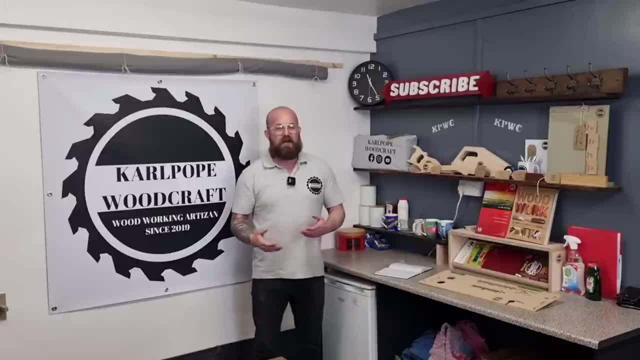 then definitely facebook marketplace again, like i said before, etsy, ebay places like that good times a year to sell the item. then mother's day is a great one for these bath caddies. last time we made these on mother's day we sold we- i think we made about 30 and we we sold them all out. and when 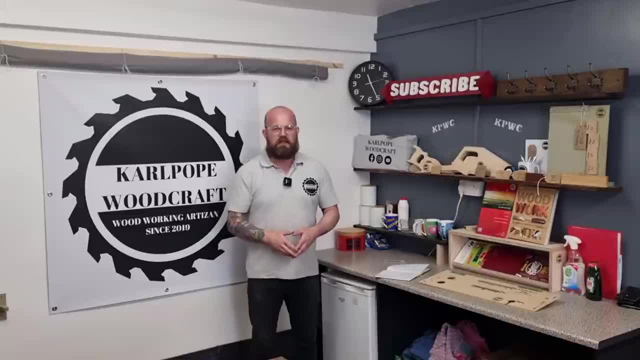 it was leading up to mother's day, we didn't we. we thought it was going to be a bit of a flop because we didn't actually sell that many and then in the last couple of days coming up to mother's day that we sold a lot. people was just picking them up left, right and center. so we saw that mother's 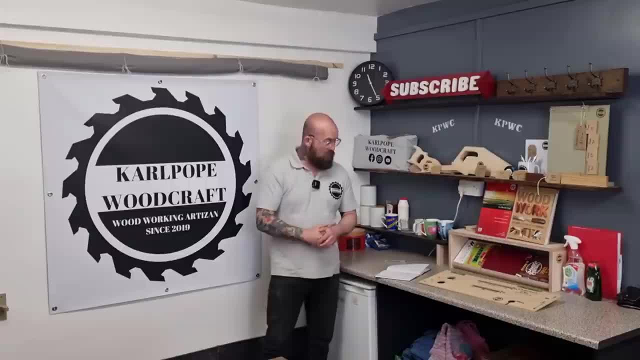 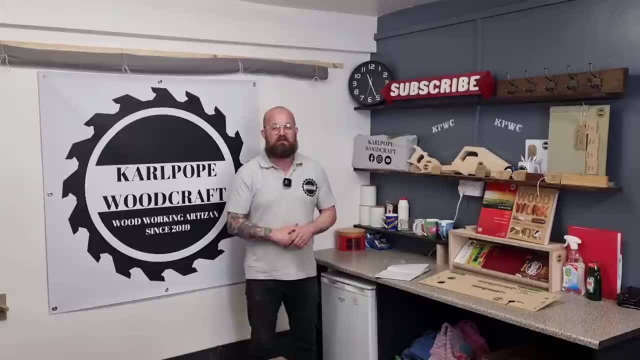 day is a great time a year for them. valentine's day would be a good one, and birthday is christmas, so anytime there's an occasion, these are a good item people are looking at. you know, handmade gifts to give for the, the loved ones, uh them, special occasions. a great time of year for these. next, 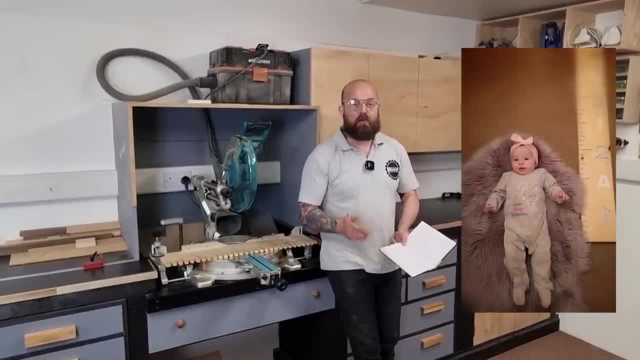 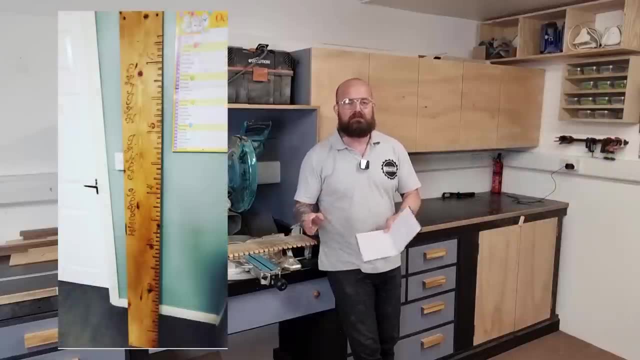 time we're going to look at is one of my personal favorites. it's the height chart, and one of the best things about this item is you can personalize it. whenever you can personalize something it's, it just makes it more sellable. you can also charge a little bit extra for having it. 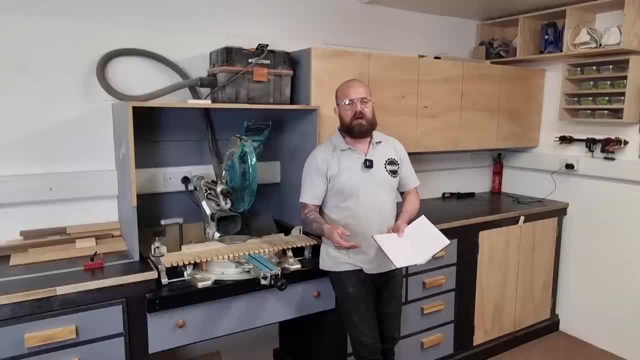 personalized. you know it's something you could do. some people charge per letter for the name when you're going to be hand routing these. we don't personally do that. we just charge a set price for the, for the entire item. again, you can finish these in different ways and make them out. 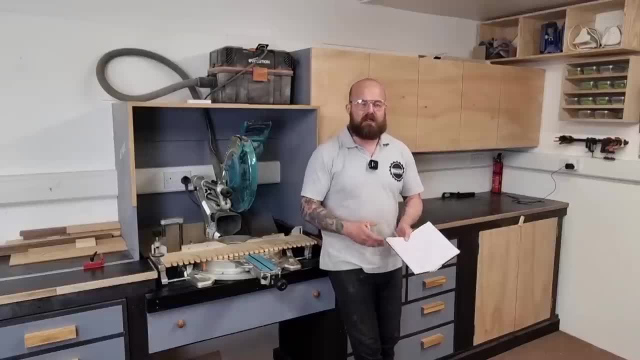 of different material and that will vary the price. you can paint them, you can varnish them and you can, just you can. you can make them your own custom to what you're looking for. so that's that's, that's what, to what you want and what your customer wants. when's a good time to sell these and 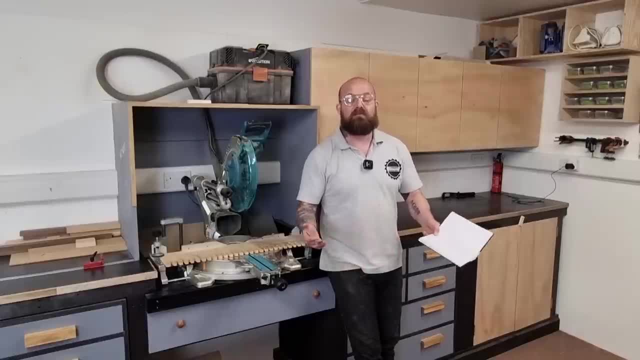 they're great for new arrivals, obviously new babies in the family. when people are thinking of a gift for a new, a new arrival, you know height chart custom, you know it's a great idea. uh, children's birthdays, you know, once they're at that sort of like toddler age and people are 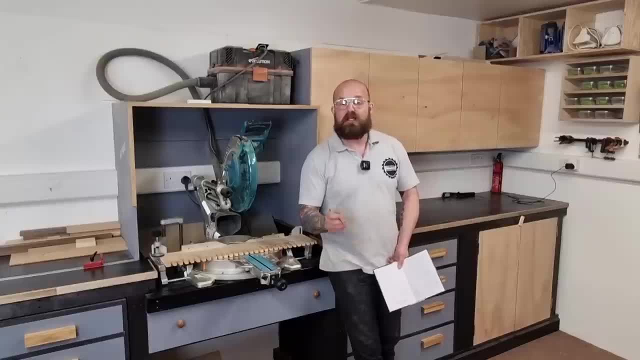 wanting to you know, keep a record of how fast they're growing. and another one is christians. christians- a great time to give as a gift. it's original and some some are different, especially when it's personalized. what are you going to need to make this then? you're going to need a router with a template. 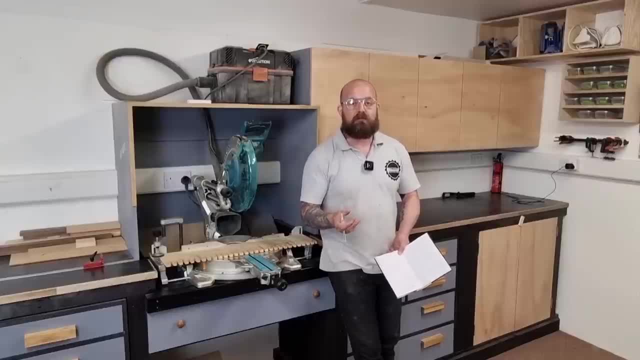 bit on and probably like an up spiral bit or straight cut bit. you want to need a cheap palm router. you don't need to spend a lot of money on these. we, we used our katsu router to make our first few ones of these. i'm going to need a saw of some type. uh, handsaw, mitre saw, again jigsaw. 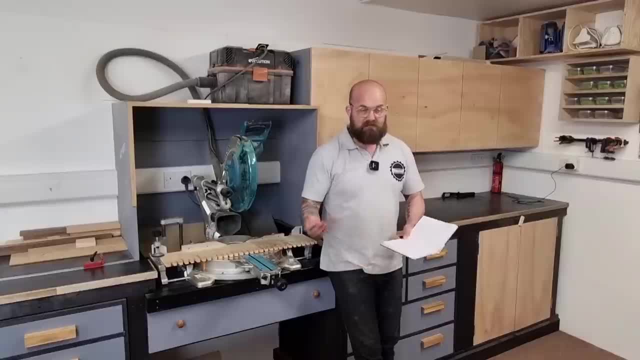 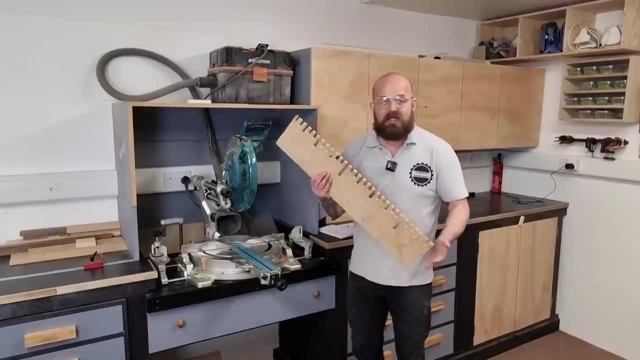 uh, not, you don't need anything fancy. uh, some form of sander. and again, templates. so if you're going to be mass producing it, you're going to need it. there are a lot of different types of little want a template. you can make these without a template just by using a speed square and running. 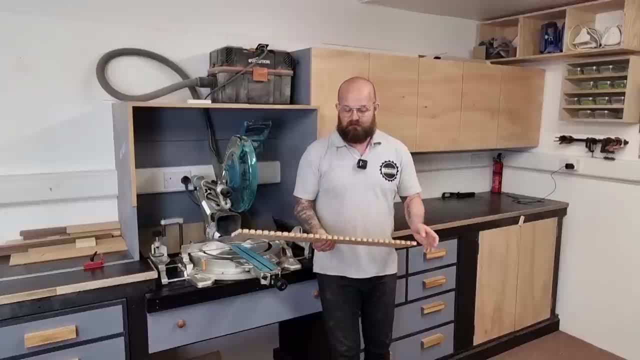 your router along the edge and doing lots of accurate marking out, but it's definitely worth making one of these. probably going to take you about an hour, if that, to make one of these. i made this one. this is the very first one i made and this was made just using a jigsaw, so no fancy. 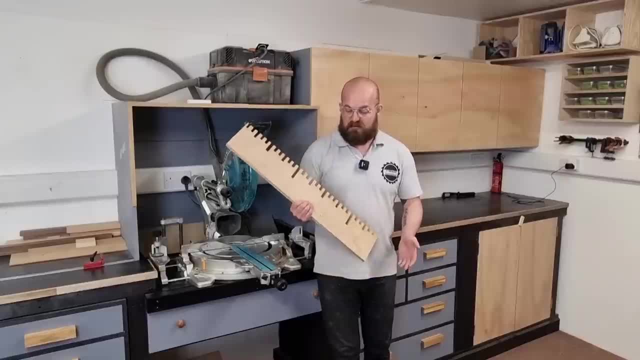 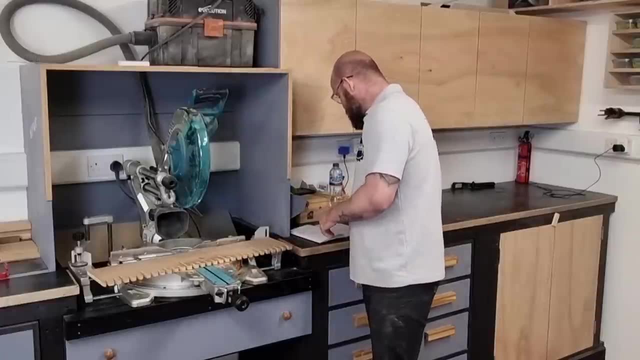 tools, took my time marking everything out, cut it out of a jigsaw and i've still used this one today. price-wise, then, how much did we say these go for j? these are generally selling at about 45 pounds, so they're quite a good seller for what they are. one board again, depending on the type of 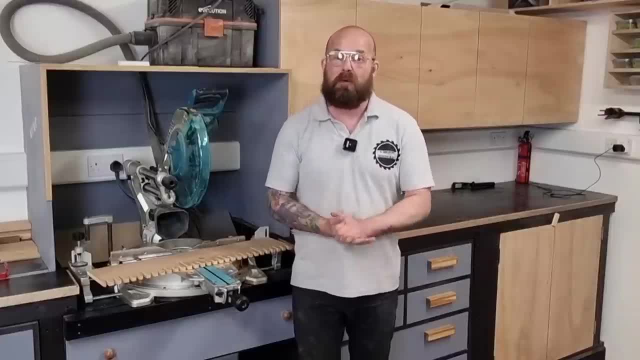 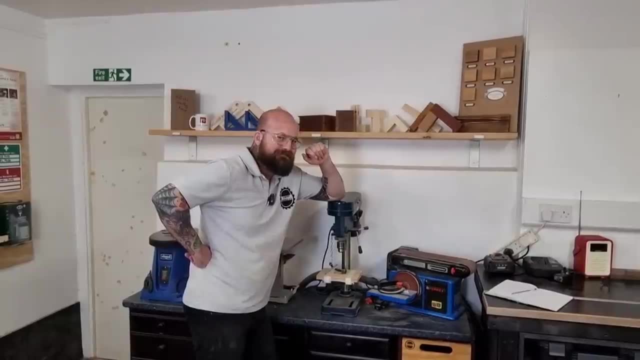 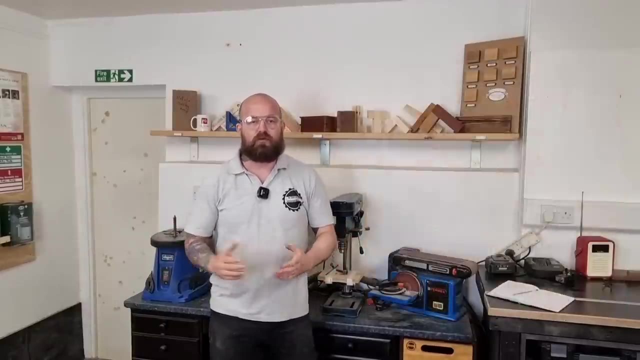 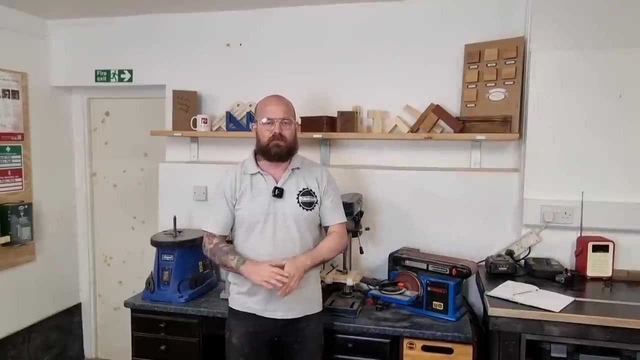 finish and the type of material that might go up by 10 pounds and down by 10 pounds in your area- radiator shelves. when would you sell these all year round? they're a. they're a really good all-round seller for the whole year. every time we advertise these on facebook marketplace- these are paid ads, by the way- we 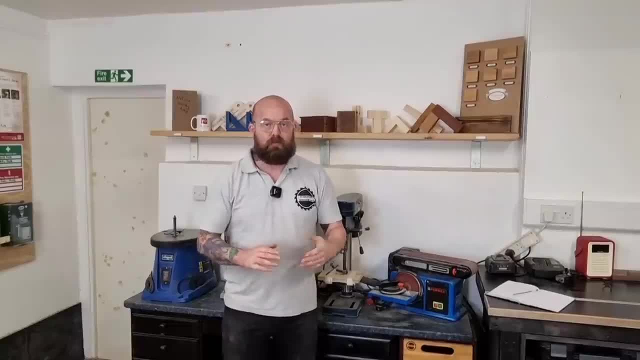 just place them on there. they do really well. we generally wait till we've got about five or six orders and then we'll go out and fit these all in a one air. the type of tools that you're going to need for the this and really simple again, you're going to see a pattern in the types of tools that. 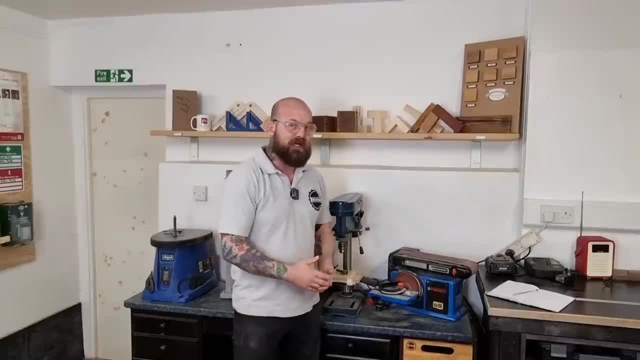 you need for these items and the reason behind this is because these are the tools we had at the time and again, it's a router, it's a handsaw, it's a sander. again, you can use different types of materials, which is going to vary the cost. you can do from oak. you. 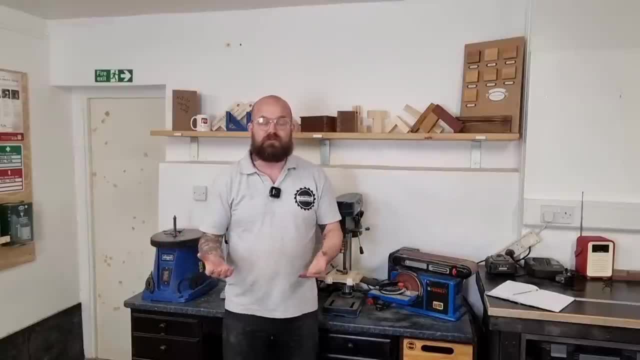 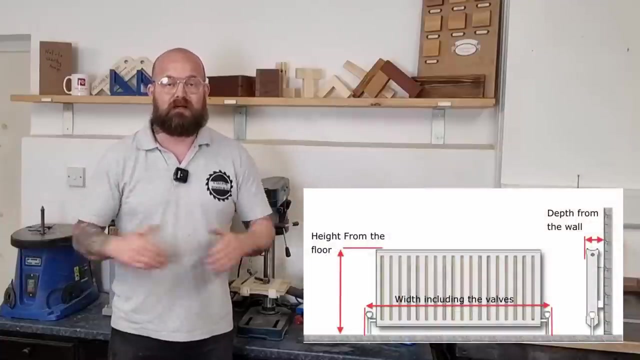 could do from walnut, it's going to put the price right up. or you could just do them out of a piece of spruce, a piece of pine board, construction timber. generally we sell ours for about 95 pound. we get the customer to send us the dimensions of the radiator from pipe to pipe at the furthest end. 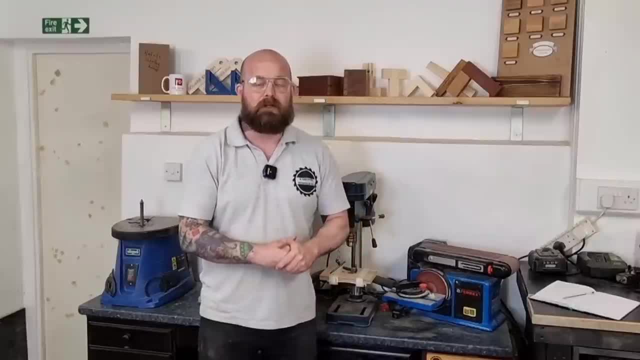 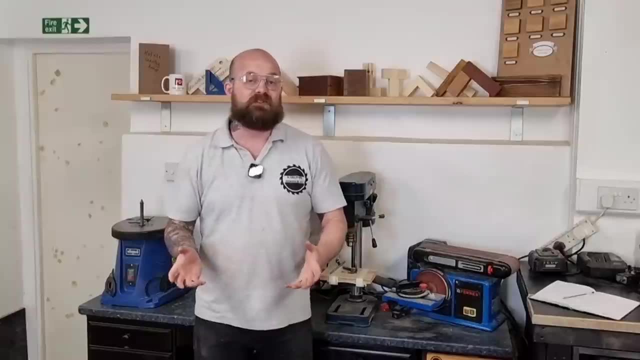 and then the depth. that way we don't have to go up to the customer's house to measure up, and then, if the customer wants us to fit them, we have an install fee of 15 pounds, and if they want to fit them themselves, we'll just drop them. 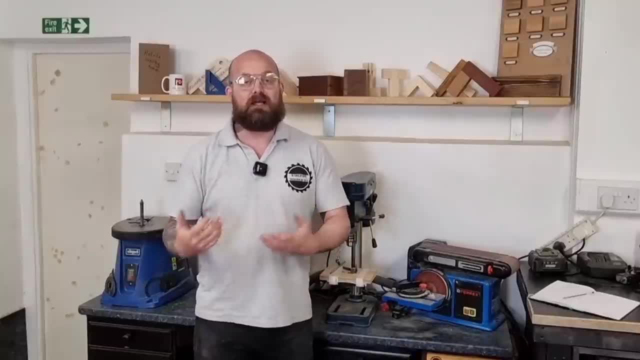 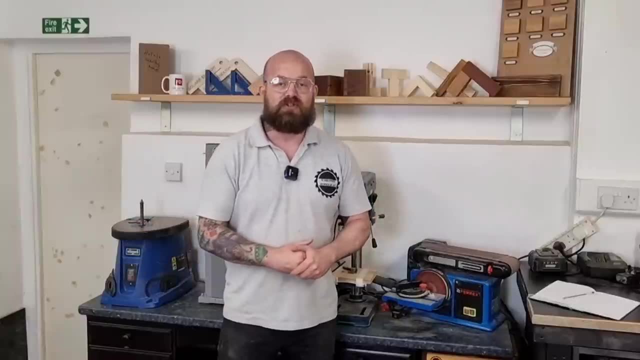 off at the house. we use hairpin legs for these, and when you buy hairpin legs you buy them in packs of four, because obviously they're designed for tables or desks or whatever. you only need two for the for the radiator shelf, and then you've got two for the next one- really easy to install. 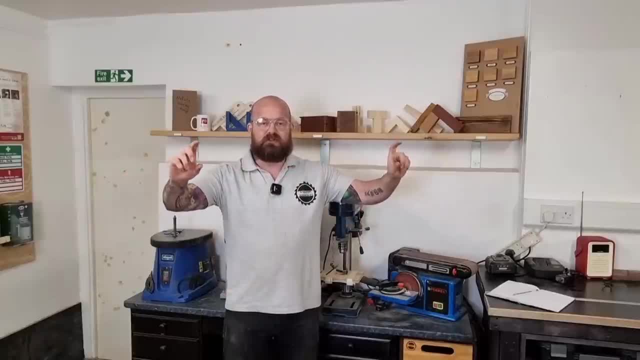 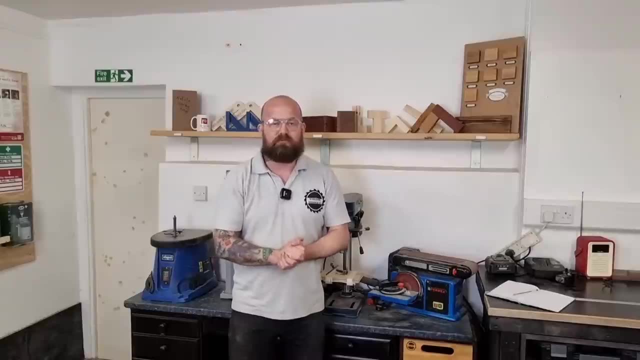 all we have is a baton along the back which is attached to the shelf. we drill a couple of holes into the wall, so you're going to need a combi drill so you can drill into brick or breeze block, and then we attach that to the wall and it's as simple as that. 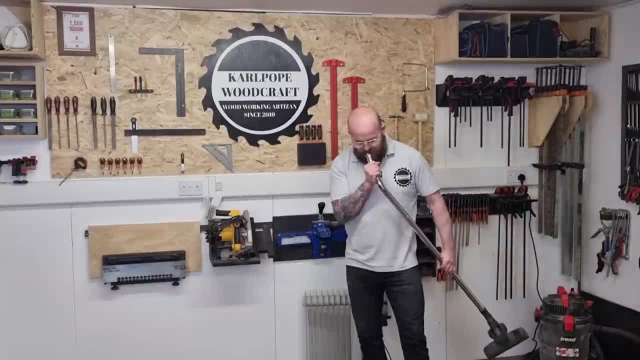 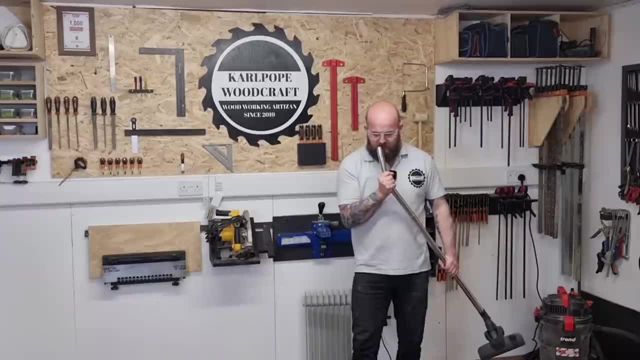 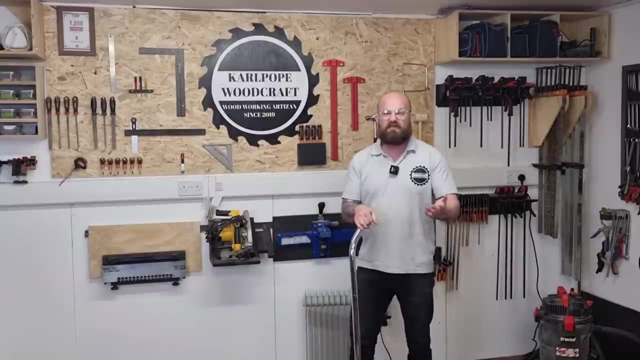 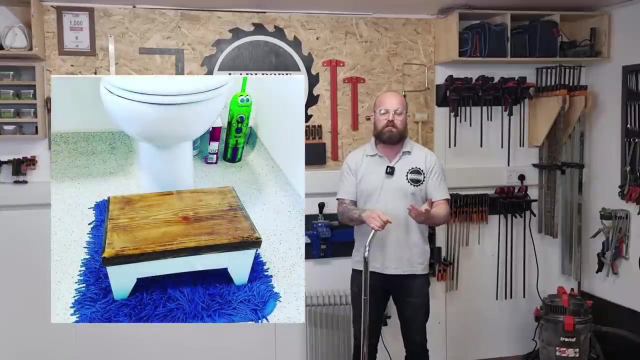 when will i, will i be famous? i can't answer that. i can't answer that. when will i see my picture in the paper? right then, moving on to the next one: stepstool. uh, stepstools- again relatively easy to build. we've got a cool video of actually me and jake doing a little challenge against each other. i make a fancy one. 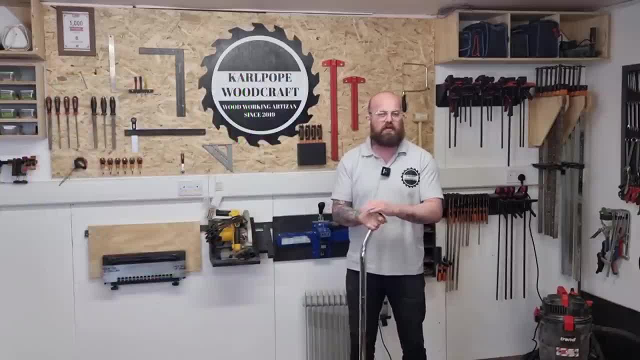 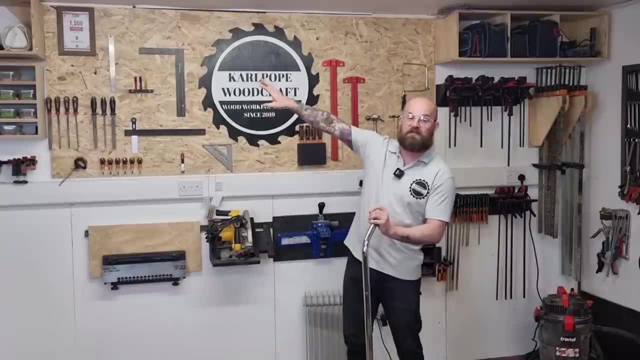 out of oak and some other hardwoods and use some you know, more complicated joinery. jacob makes his out of a pocket hole joinery and we use that in the workshop because jacob can't reach these high shelves up behind me so he needs to use that to step up to get up there. 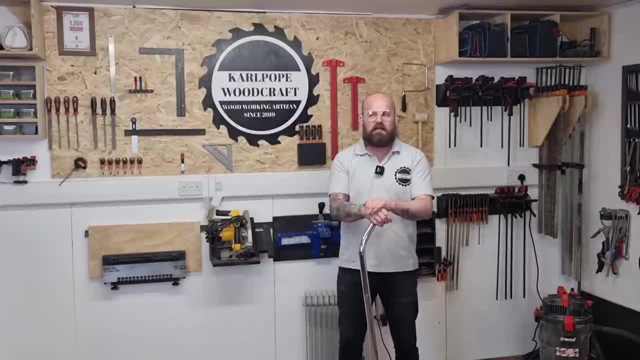 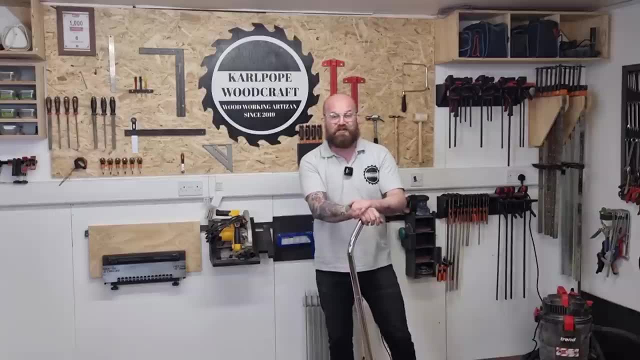 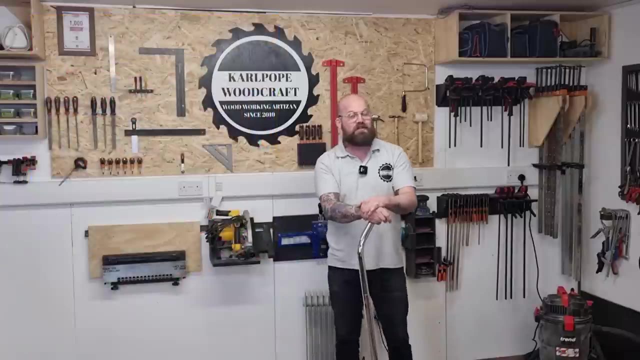 stepstools are great again for young ones especially and people who are a. what's the word i'm looking for? yeah, yeah, that's the one: height impaired. so people who are height impaired, like my wife, who can't reach up to the top shelf in the cupboards. so i made one for my wife for christmas. 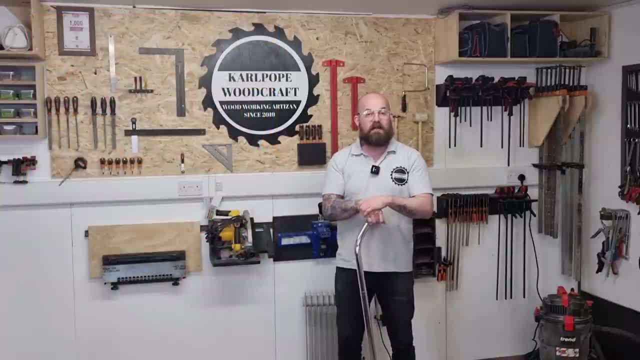 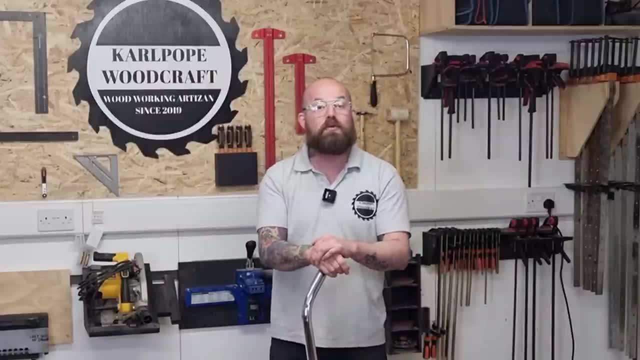 and they're also great for, you know, children so when they when the the toilet, training so for little boys stepping up to have a wee in the toilet and also helping to wash the pots and do chores around the house, reaching the side. so they're a great little gift for young ones and 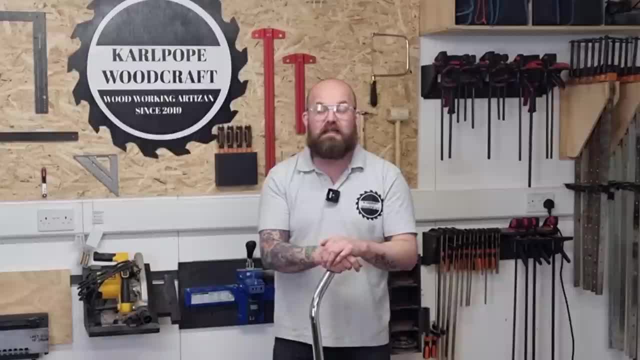 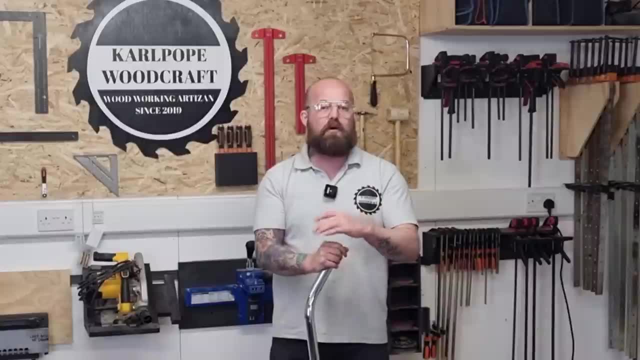 people who aren't very tall need to reach things. uh, simple to make, the one that jacob made was used with pocket hole joinery and it's super strong. so again, uh, for that one we used a pocket hole jig, so you're going to need one of those. 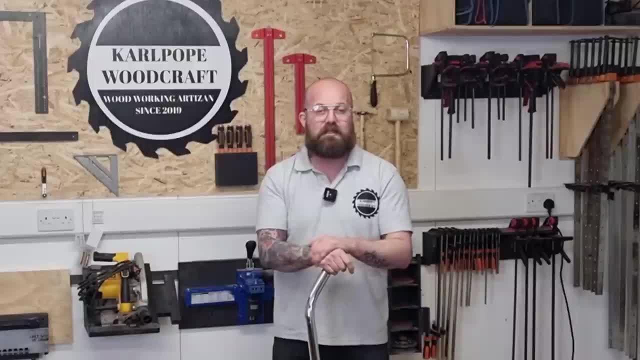 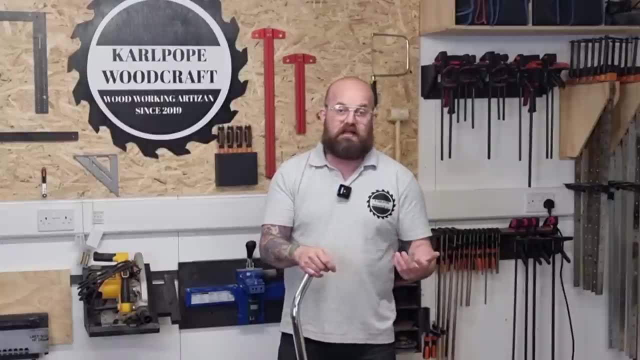 uh, but you can get them for as cheap as about 10 or 15 pounds, all the way up to the, you know, the more fancy ones like like the ones that we use. what else would you need? you'd use? you'd need a saw, a sander and a router if you want to put a nice trim around the edge of chamfer or a roundover. 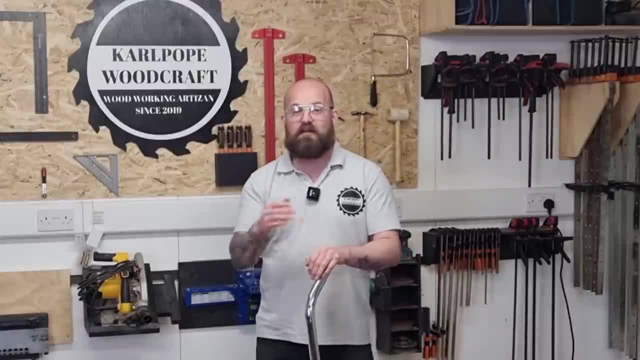 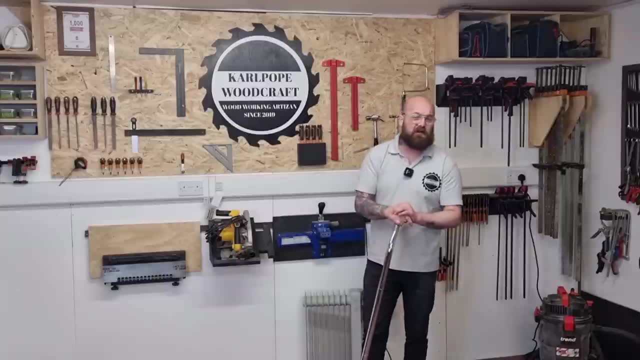 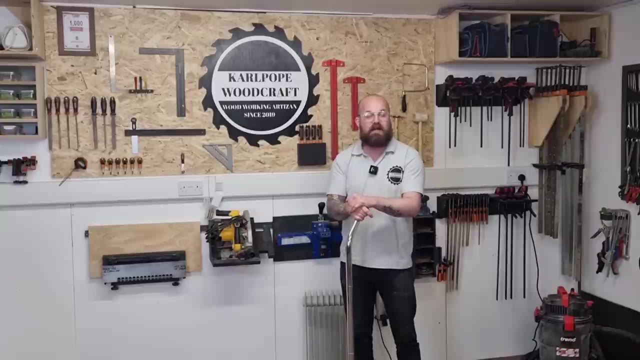 and again material: wise pine, any anything up to oak, or any nice hardwoods that you want to use. the step stools sell then for about 25 pounds, and it all depends again on the finish and the materials you're using. the next item, what we're going to look at then, and the final item, is just: 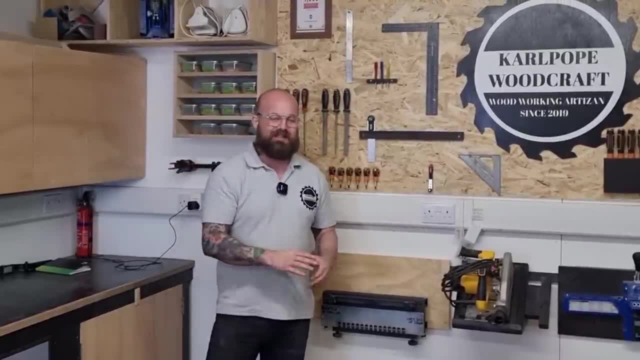 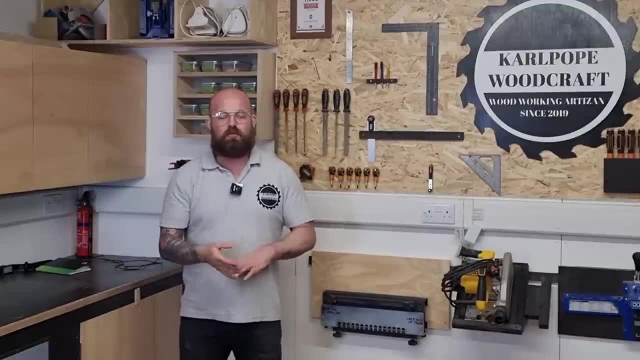 before we go on to the last item, then guys are just going to give you a couple of little tips on selling the item. when you, when you upload this onto your facebook marketplace, you want some some nice pictures. so, whatever you make, put it up in your house first, or in your bar, or with your child. 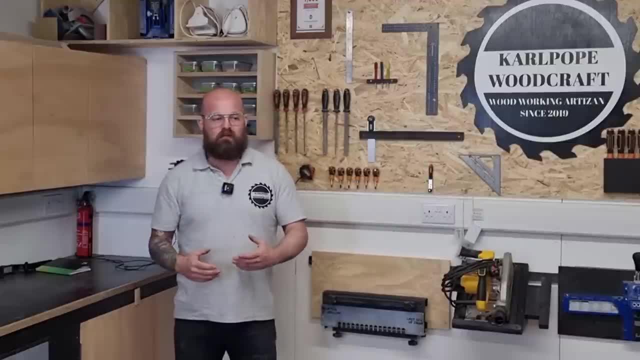 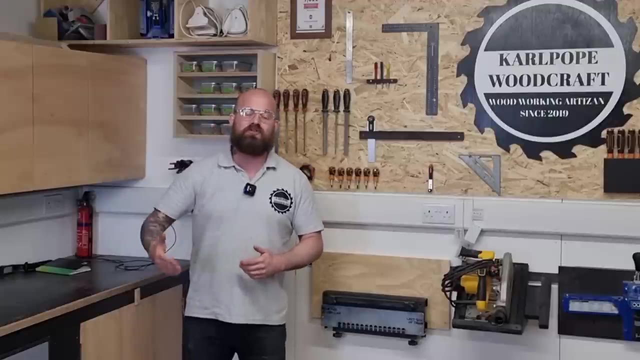 chart or something like that. just take some nice pictures, uh, give a good description of the item, the materials, the size, the dimensions. try and cover as many bases as you can. if you don't do this, you're going to get inundated with questions and you're going to get the same question over and 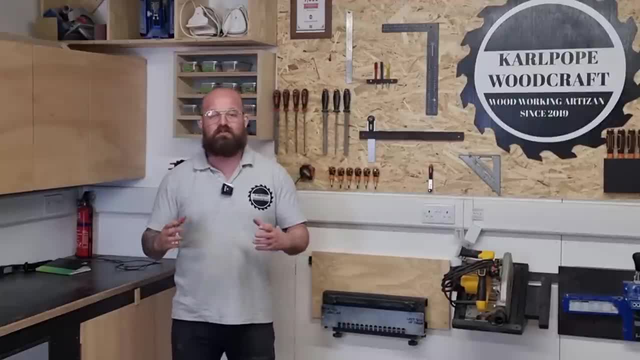 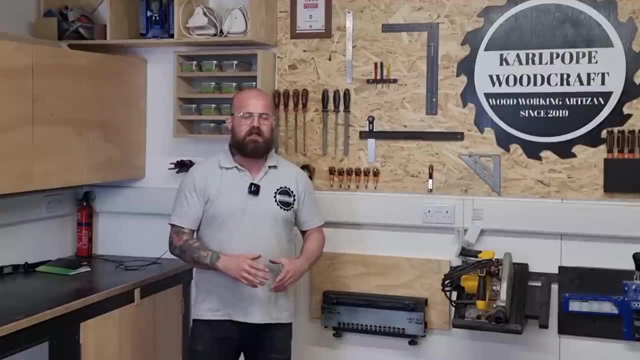 over again. how big is it, how wide is it, how high is it? so if you try and cover all these areas, especially the dimensions and the materials, then you'll get less time wasters. but if you are a beginner, you can just take some of the extra parts and just keep on going. 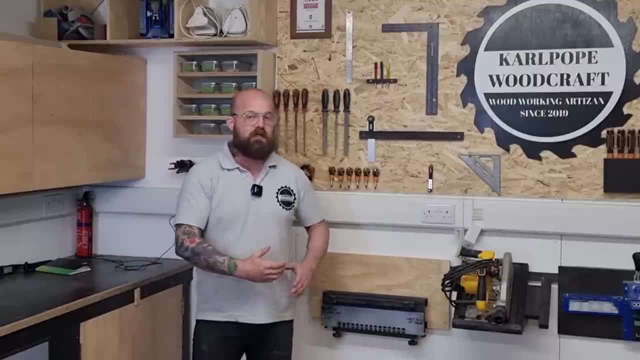 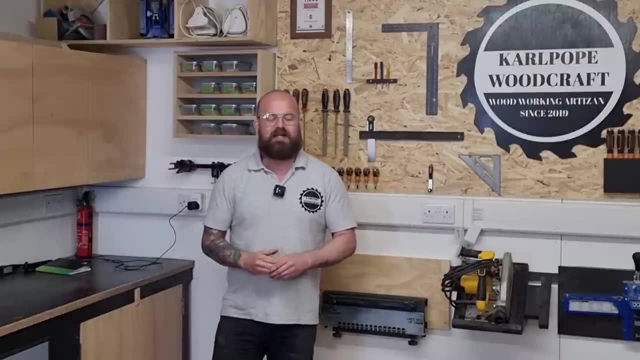 and then if you want to make more money, you can just go to the link in the description. so just keep on getting the details of the items and you'll just have to make a couple of nice pictures to help it sell and upload it to as many places as you can. the more you can get it out there. 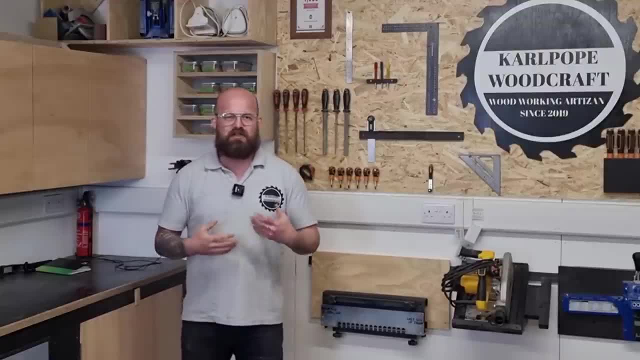 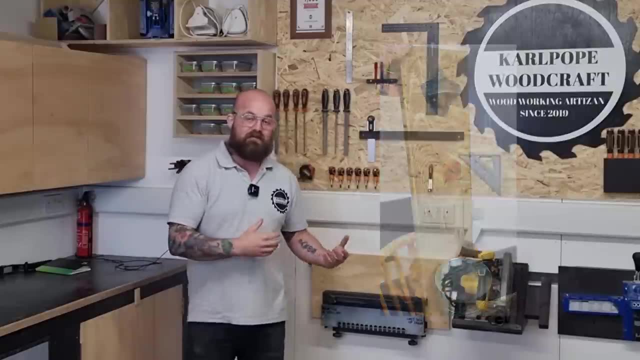 even if you pay for a small promotion, maybe. uh, the more people are going to see it, the more people that see, the more sales you're gonna make. right then on to the last item. the last item is a beer bottle opener, and these are great for father's day, uh, birthdays, uh, christmas great. 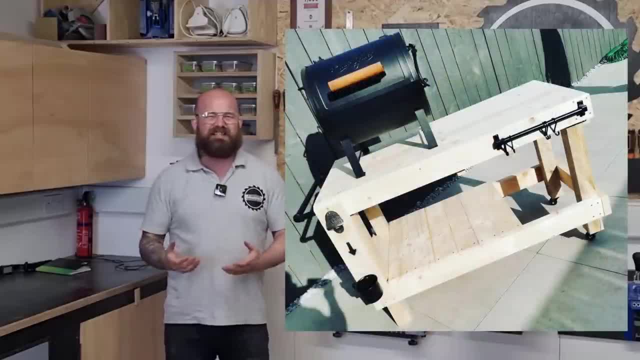 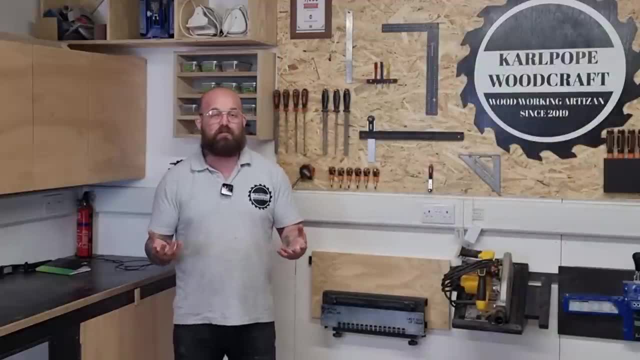 garden for in the summer. just really easy to make. all you need is a saw and a drill, really, and a bit of sandpaper. you can finish them in any different way you want. if you're using reclaimed timber, you can get your blowtorch on there and just give them a light burn and then a light sand. 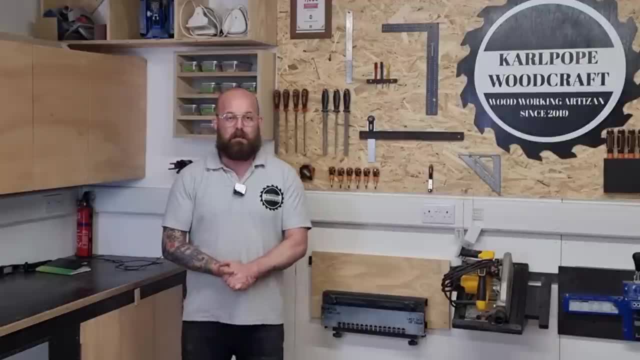 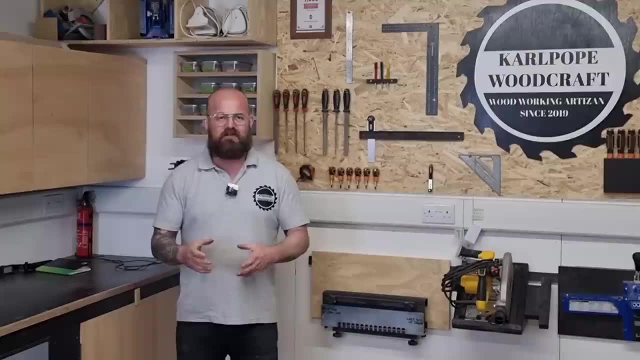 a spray, a bit of polyurethane on there, a bit of wax, dead simple. we generally put a little metal cup and we go to places like pound shop, pound land, and in the summer they sell these little metal buckets for for plants and they're normally a pound for a couple and you can just screw them.